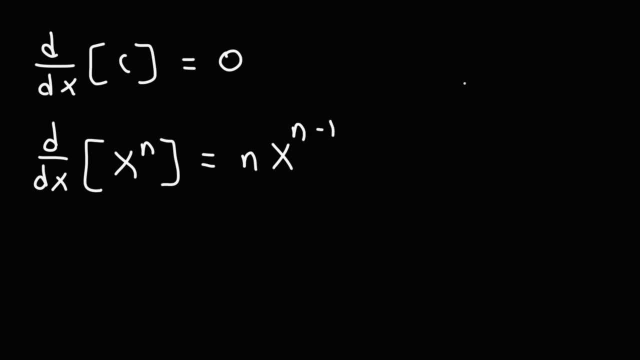 raised to the n-1.. So, for instance, the derivative of x cubed is 3x squared. The derivative of x to the fourth is 4x cubed. The derivative of x to the fourth is 4x cubed. 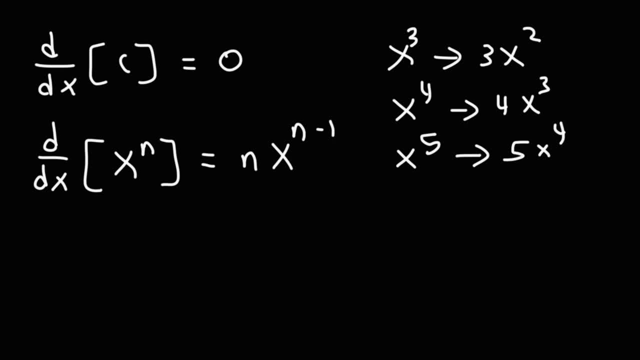 The derivative of x to the fifth is 5x to the fourth. So that's how you can employ the power rule to find derivatives of functions like this. Now, instead of having a variable raised to a constant, what if we have a constant raised to a variable? The derivative of a to the x is going: 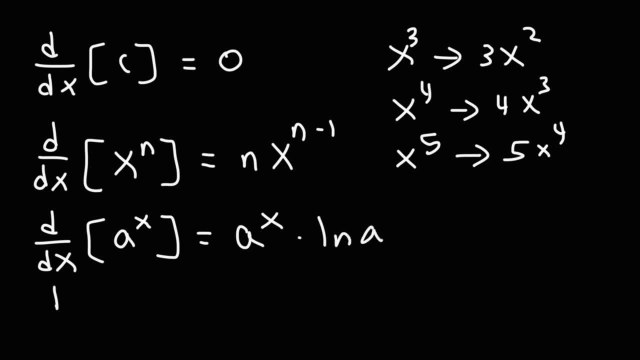 to be a to the x times ln a. Now the reason why we get that is because the derivative of x is 1.. But let's say we have the derivative of a to the u, where a is a constant but u is a function of x. This is going to be: 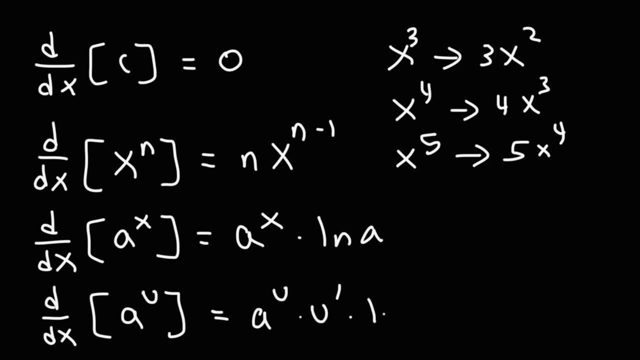 a to the u times, the derivative of u times, ln a- Here we would have the derivative of x, but that's just going to be 1.. Now, if you ever get this- the derivative of a variable raised to a constant or the derivative of a variable raised to a variable- this, rather than having a formula- you need to employ a process called logarithmic differentiation, and I have a video on YouTube that covers that. So if you go to the YouTube search bar and type in logarithmic differentiation, organic chemistry tutor, you should see a video that will come up and explain how to do problems like this. 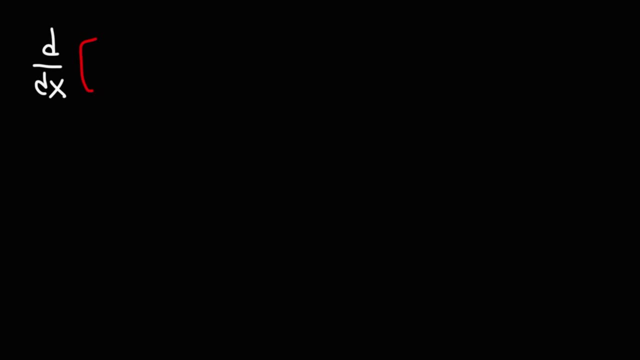 Next up, we have something called the constant multiple rule. So if you have, if you're trying to find the derivative of a function multiplied by some constant c, it's simply going to be that constant times the derivative of that function. So for instance, let's say, if we want to find the derivative of 5x to the 4.. 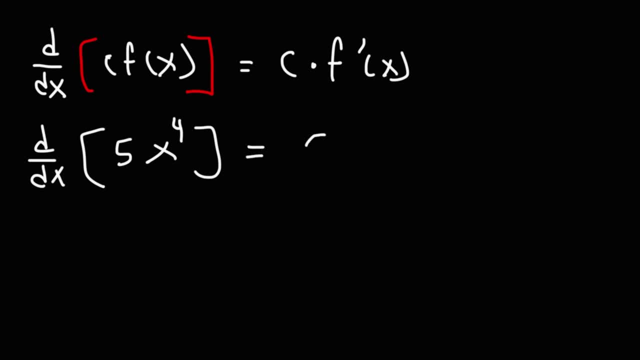 We know the derivative of x is going to be 5x to the 4.. But we can rewrite this as 5 times the derivative of x to the 4th And using the power rule, we know this is going to be 5 times 4x cubed, which becomes 20x cubed. 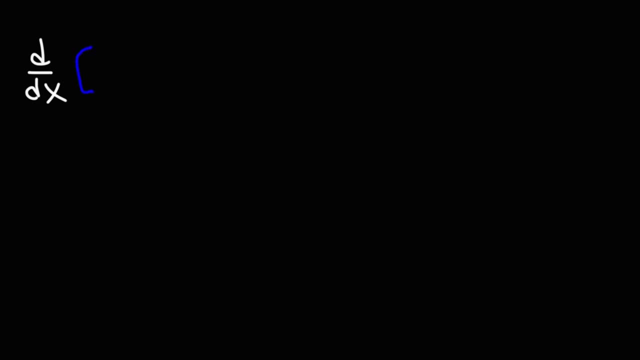 The next formula you need to be familiar with is the power rule. So if we have two functions, u and v, and they're multiplied to each other, the derivative of x to the 4th is going to be 5x to the 4th. 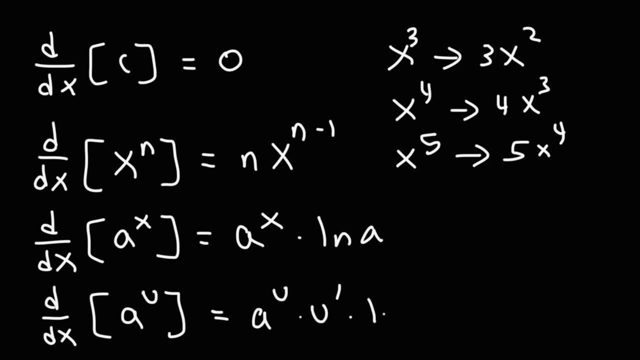 a to the u times, the derivative of u times, ln a- Here we would have the derivative of x, but that's just going to be 1.. Now, if you ever get this- the derivative of a variable raised to a constant or the derivative of a variable raised to a variable- this, rather than having a formula- you need to employ a process called logarithmic differentiation, and I have a video on YouTube that covers that. So if you go to the YouTube search bar and type in logarithmic differentiation, organic chemistry tutor, you should see a video that will come up and explain how to do problems like this. 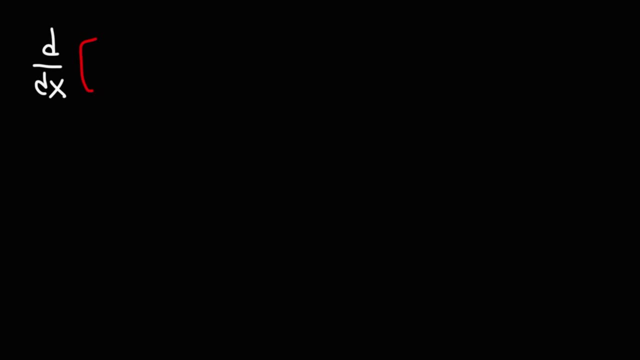 Next up, we have something called the constant multiple rule. So if you have, if you're trying to find the derivative of a function multiplied by some constant c, it's simply going to be that constant times the derivative of that function. So for instance, let's say, if we want to find the derivative of 5x to the 4.. 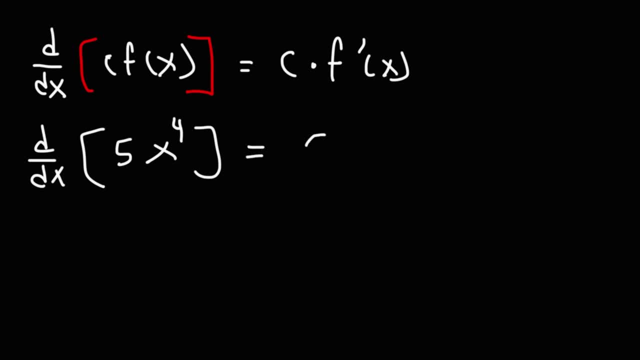 We know the derivative of x is going to be 5x to the 4.. But we can rewrite this as 5 times the derivative of x to the 4th And using the power rule, we know this is going to be 5 times 4x cubed, which becomes 20x cubed. 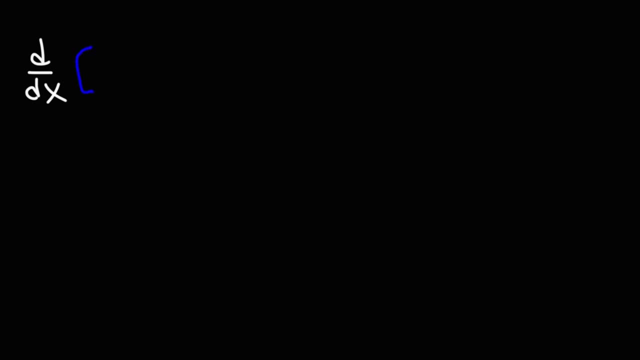 The next formula you need to be familiar with is the power rule. So if we have two functions, u and v, and they're multiplied to each other, the derivative of x to the 4th is going to be 5x to the 4th. 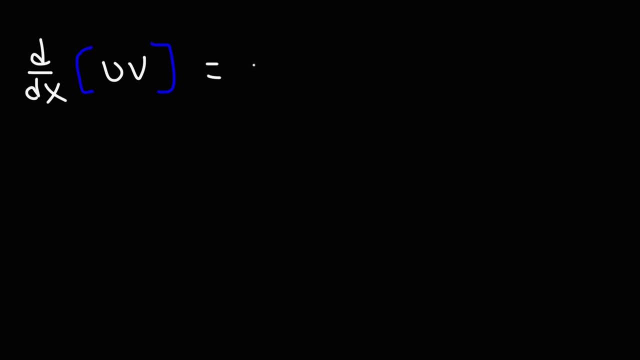 So the derivative of the product of these two functions is going to be u'v plus uv' So it's the derivative of u times, v plus u times, the derivative of v. Next up we have the quotient rule. So here we have a fraction of two functions or a division of two functions. 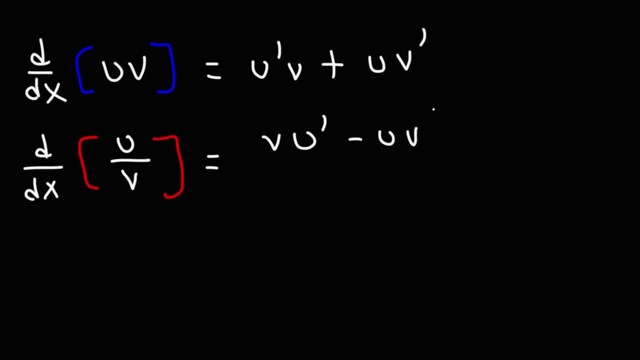 And it's going to be 5x to the 4th, And it's going to be v u' minus u v' over v squared. So that's the formula associated with the quotient rule. Now, sometimes you may need to find the derivative of a composite function. 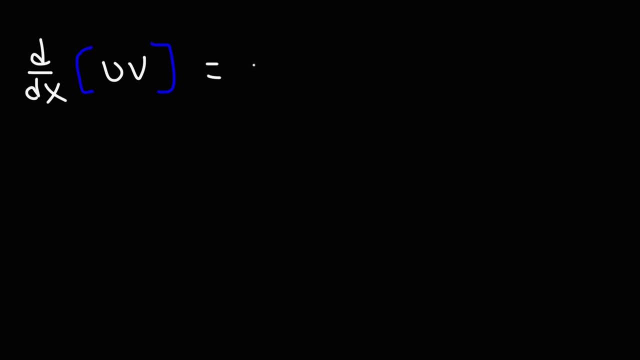 So the derivative of the product of these two functions is going to be u'v plus uv' So it's the derivative of u times, v plus u times, the derivative of v. Next up we have the quotient rule. So here we have a fraction of two functions or a division of two functions. 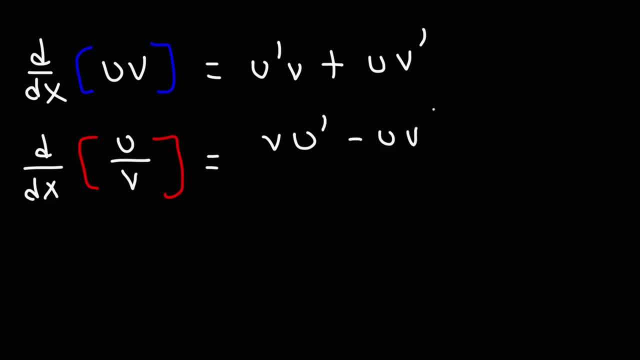 And it's going to be 5x to the 4th, And it's going to be v u' minus u v' over v squared. So that's the formula associated with the quotient rule. Now, sometimes you may need to find the derivative of a composite function. 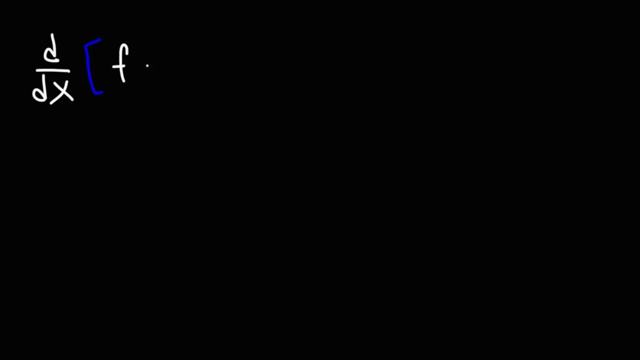 In this case you need to use a chain rule. So let's say we have f of g of u. We want to find the derivative of that. So let's say we have f of g of u. So first we're going to find the derivative of the outer function f, we're going to keep. 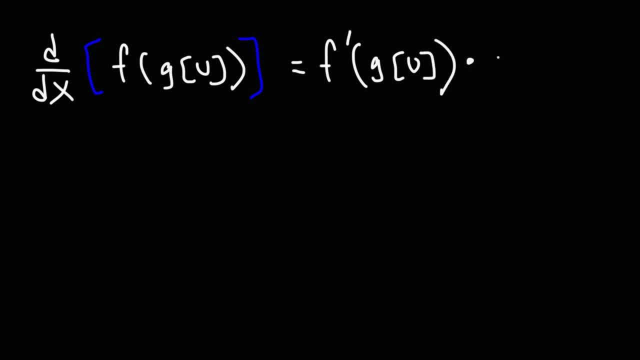 the inside part the same, and then we're going to multiply it by the derivative of the inside part, That is, the derivative of g, And then we'll multiply it by the derivative of the inside of g, which is u, so that will. 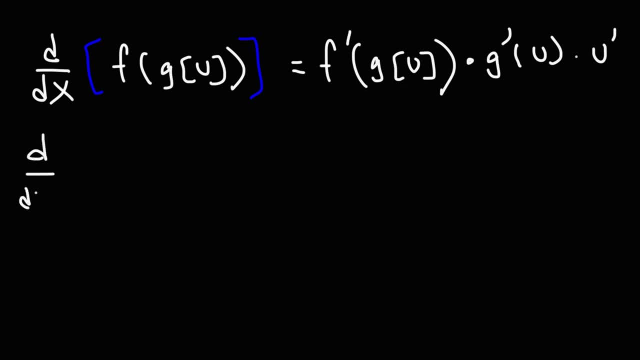 be times u prime. Now you might see the chain rule represented as a function of x instead of u. so let's say, if you have this f of g of x, It's going to be the derivative of the outside function. we'll keep the inside part the same. 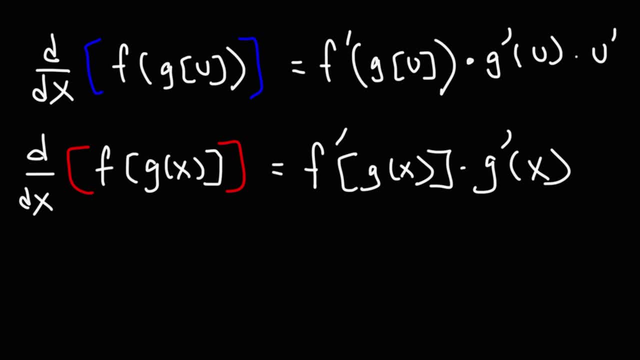 and then times the derivative of the inside function. Now the derivative of x is 1, so there's no point in writing that it would just be times 1.. So if you have x, this is all you need. But if you have a function u or a function like where u is a function of x, you're also. 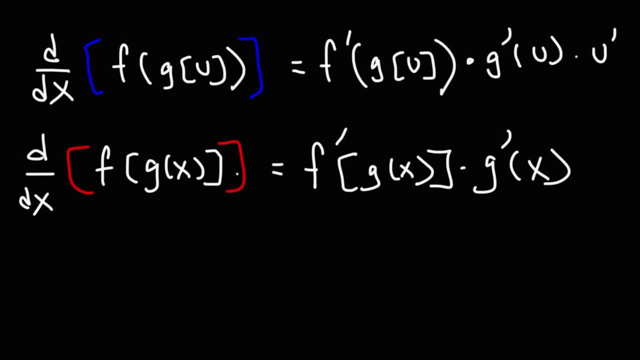 going to have u prime at the end, So keep that in mind. So you've got to differentiate the outer function f, and then work your way towards the middle, Then g and then u. Now for those of you who want additional example problems on this, check out the links in the. 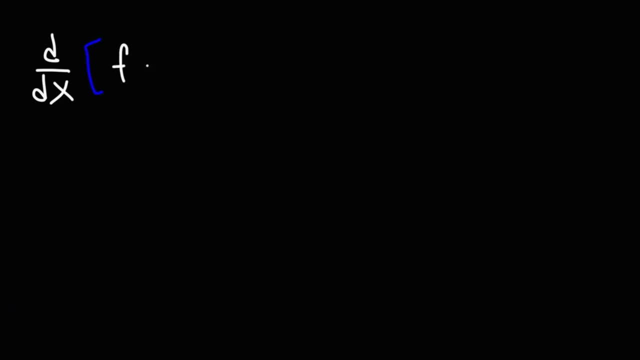 In this case you need to use a chain rule. So let's say we have f, of g, of u And we want to find the derivative of that. So first we're going to find the derivative of the outer function f. 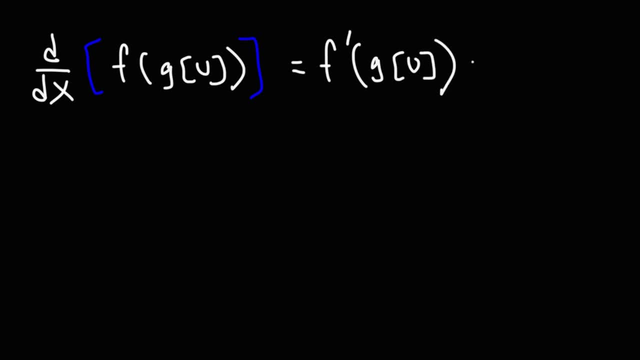 We're going to keep the inside part the same, And then we're going to multiply it by the derivative of the inside part, That is, the derivative of g, And then we'll multiply it by the derivative of the inside of g, which is u, so that will be times u'. 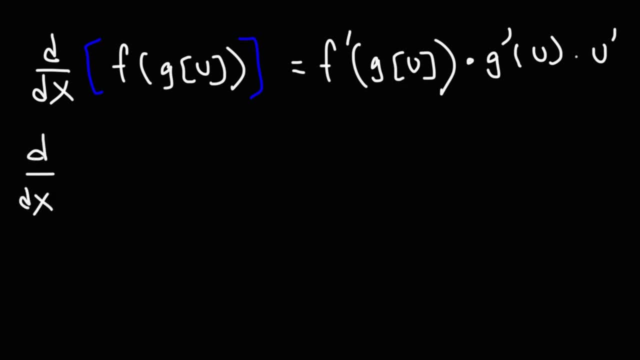 Now you might see the chain rule represented. in this case It's represented as a function of x instead of u. So let's say, if you have this f, of g, of x, It's going to be the derivative of the outside function. 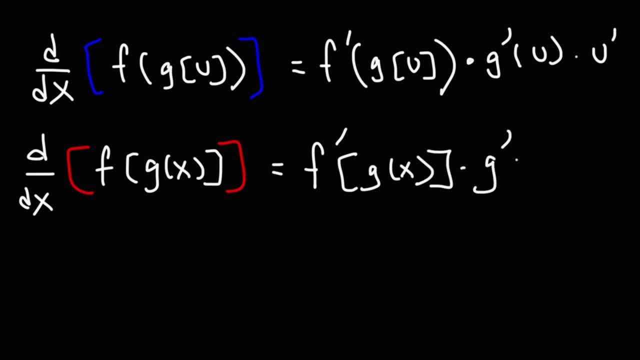 We'll keep the inside part the same And then times the derivative of the inside function. Now, the derivative of x is 1, so there's no point in writing that It would just be times 1.. So if you have x, this is all you need. 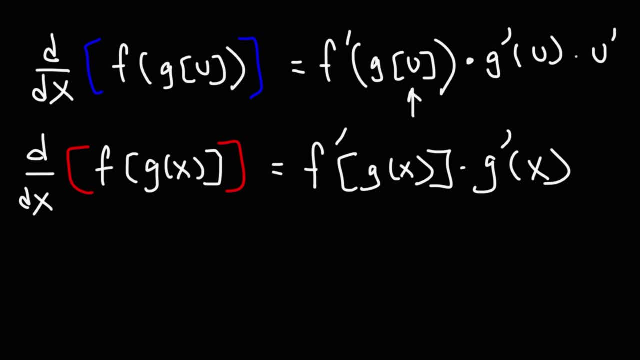 But if you have a function u or a function like or use a function of x, you're also going to have u' at the end, So keep that in mind. So you've got to differentiate the outer function f and then work your way towards the middle. 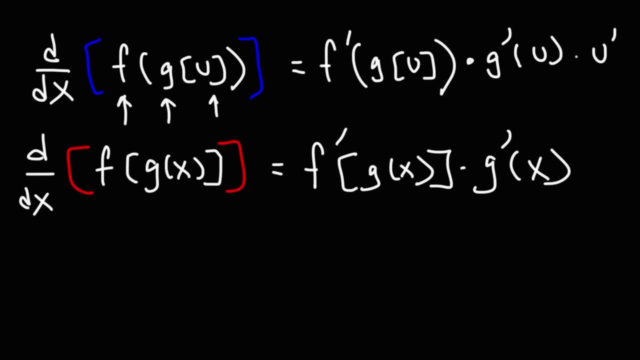 Then g and then u. Now, for those of you who want additional example problems on this, check out the links in the description section below. Now let's continue. Let's continue. Let's talk about another form of the chain rule When it's combined with the power rule. 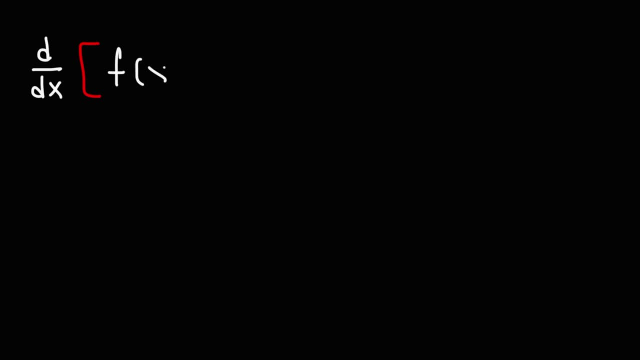 So let's say we want to find the derivative of the function f of x, But it's raised to the n. So first we're going to focus on the outside part, We're going to keep the inside part the same, So it's going to be f of x. 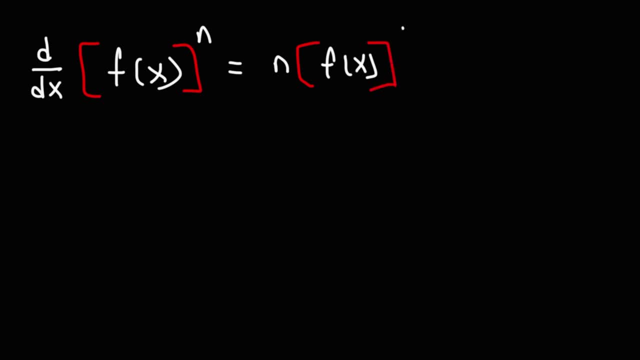 So it's going to be f of x. So it's going to be n times f of x to the n raised to the n minus 1. Much like the power rule Where it was n x raised to the n minus 1.. 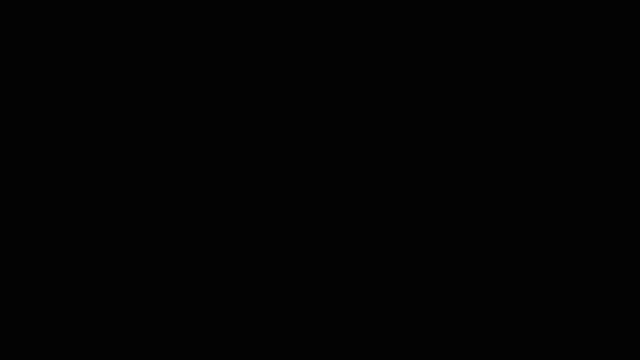 description section below. Now let's continue. Let's talk about another form of the chain rule, when it's combined with the power rule. So let's say we want to find the derivative of the function f of x, but it's raised to 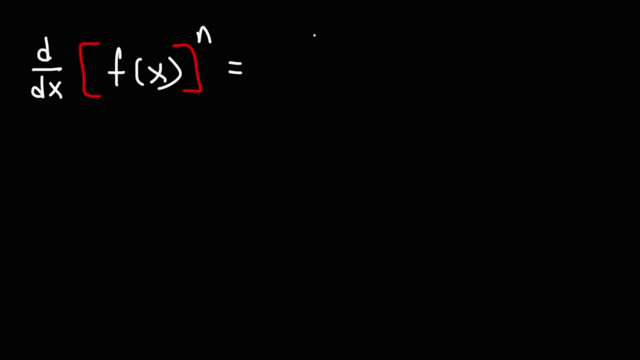 the n. So first we're going to focus on the outside part, We're going to keep the inside part, We're going to keep the inside part the same. So it's going to be n times f of x to the n raised to the n minus 1.. 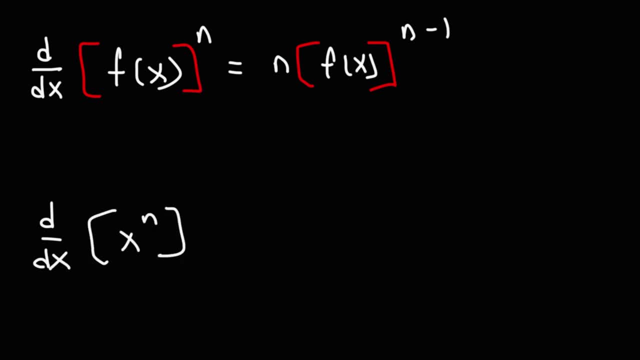 Much like the power rule, where it was n, x raised to the n minus 1.. But we do have a function on the inside. it's not just x, It's a function of x. So now we've got to find the derivative of the inside, so we're going to multiply it. 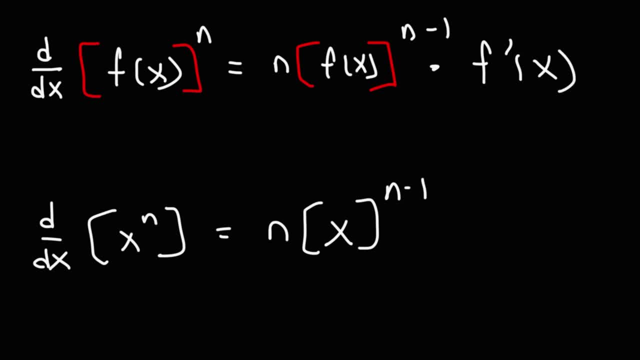 by the derivative of the inside. So this combines the power rule with the chain rule. Another formula that's associated with the chain rule is this one: dy dx is equal to dy du times du over dx. Now let's talk about the derivative of logarithmic functions. 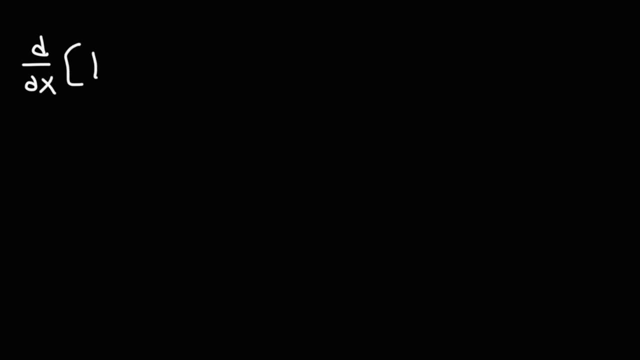 So the derivative of logarithmic functions. The derivative of logarithmic functions is the derivative of the function f of x. so let's say we want to find the derivative of log base a of u. where u is a function of x, it's going to be u prime over u ln a. 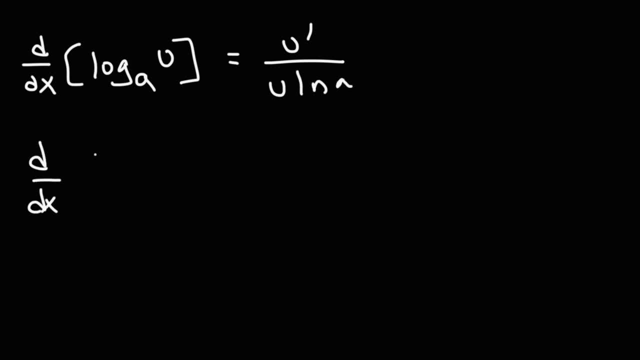 if we want to find the derivative of the natural log of u. keep in mind the base of a natural log is e. it's going to be u prime over u. it's the same as this one. the only issue is l and e is equal to one, so you can write it as just u on the bottom. so those are the two formulas you need to. 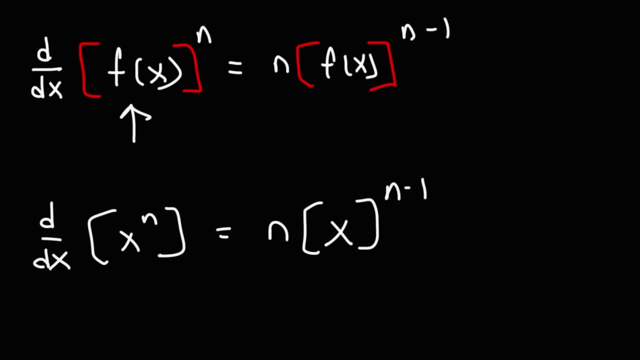 But we do have a function on the inside. It's not just x, It's a function of x. So now we've got to find the derivative of the inside. So we're going to multiply it by the derivative of the inside. So this combines the power rule. 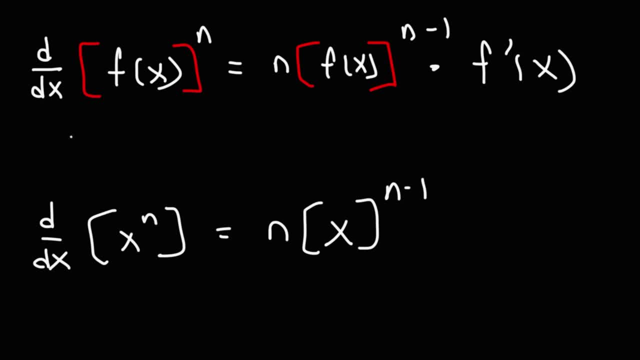 With the chain rule. Another formula that's associated with the chain rule is this one: dy dx is equal to dy du times du over dx. Now let's talk about the derivative of logarithmic functions. So let's say we want to find the derivative of log base a of u. 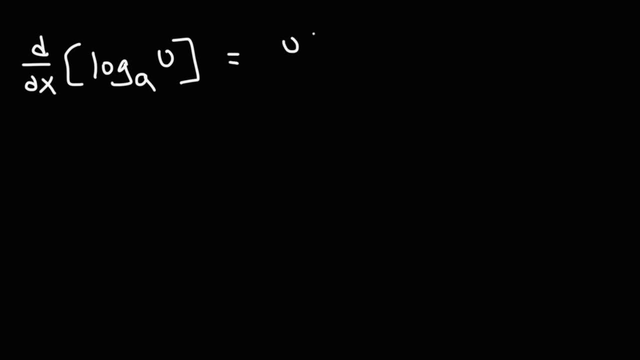 Where u is the derivative of log base a of u And u is a function of x, It's going to be u prime over u, ln, a. If we want to find the derivative of the natural log of u, Keep in mind the base of a natural log is e. 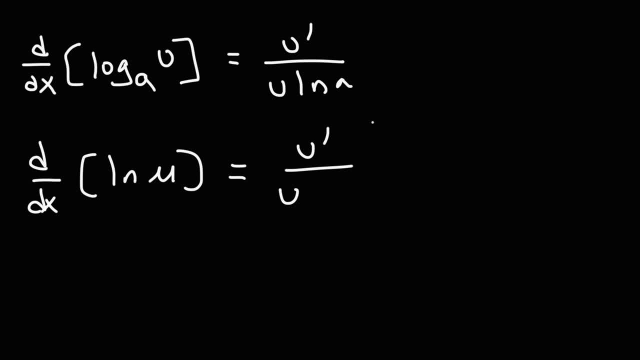 It's going to be u prime over u. It's the same as this one. The only issue is ln e is equal to 1. So you can write it as just u on the bottom. So those are the two formulas you need to be familiar with when finding the derivatives of logarithmic functions. 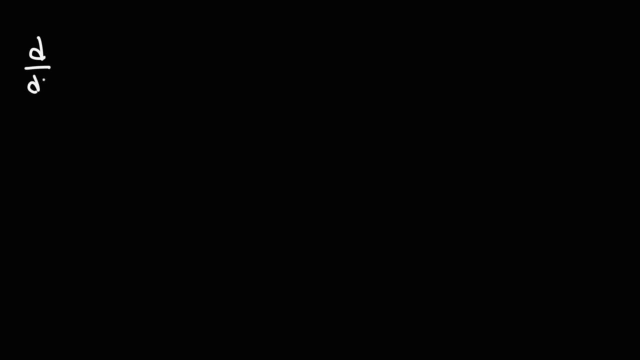 Now let's focus on trig functions. The derivative of sine of u Is going to be cosine u times u prime. Now if you just have sine x, The derivative of sine u Is simply cosine x. You can think of it as cosine x. 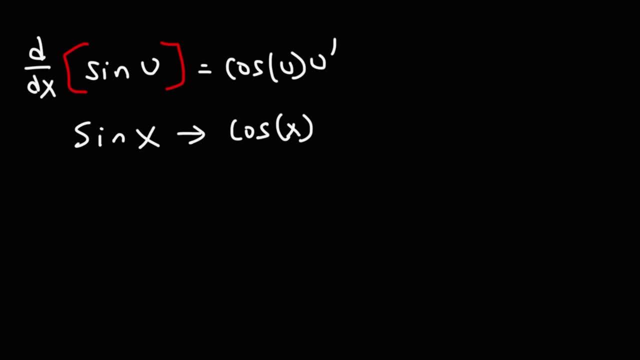 And the derivative of x is 1.. So it's just cosine x. But let's say if u was x squared, If you want to find the derivative of sine x squared, It's going to be cosine x squared And then times the derivative of x squared. 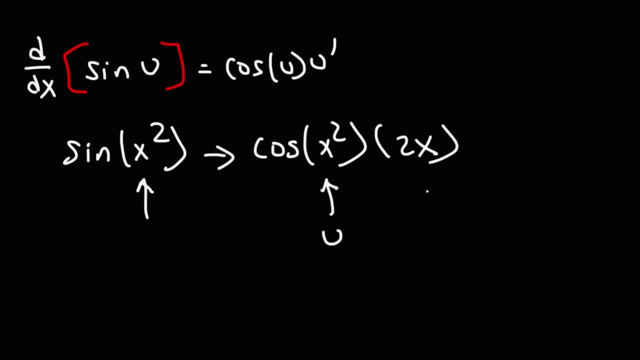 Which will be 2x. So this is the u part And this is the u prime part. That's why I like to write it in this format. It reminds you that You'll need to employ the chain rule If you have something other than x as the angle. 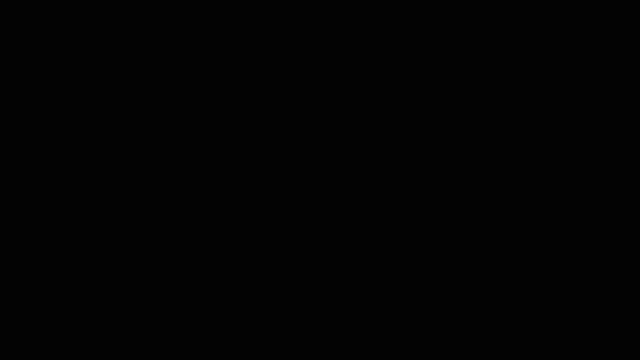 be familiar with when finding the derivatives of logarithmic functions. now let's focus on trig functions. the derivatives of log of u. the derivative of sin of u is going to be cos u times u prime. now, if you just have sin x, the derivative of sin x is simply cos x. 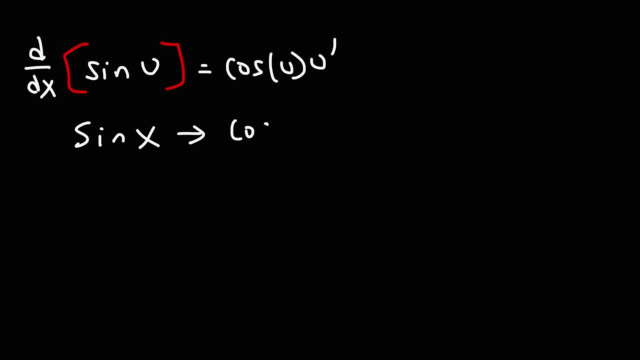 you can think of it as cos x and the derivative of x is 1, so it's just cos x. but let's say, if you've written the derivative of sin x, u was x squared. If you want to find the derivative of sine x squared, it's going to be cosine x. 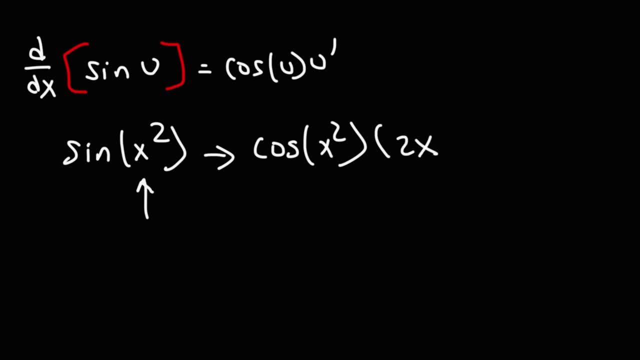 squared, and then times the derivative of x squared, which will be 2x. So this is the u part and this is the u prime part. That's why I like to write it in this format. It reminds you that you'll need to employ the chain rule if you have something other than x as the angle. 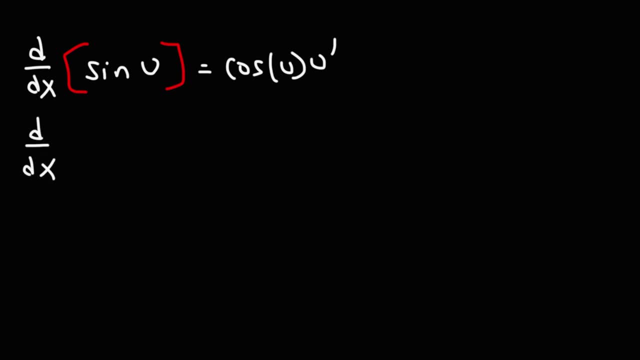 Now the derivative of cosine u. this is going to be negative, sine u times u prime. The derivative of tangent of u is secant squared. Now for cotangent, it's going to be negative cosecant squared and, as always, times u prime. 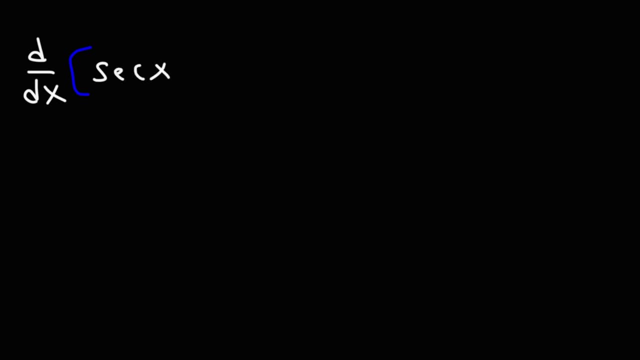 Now the next two that you need to know are the derivative of secant and the derivative of secant's cousin, or cosecant, And they're quite similar. If there's a c in front, typically it's going to have a negative sign. 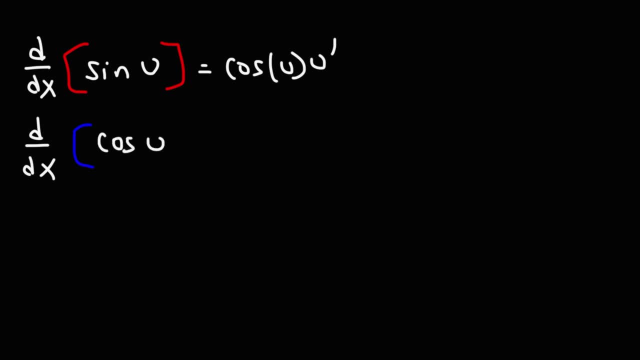 Now the derivative of cosine: u. This is going to be negative. sine U times u prime. The derivative of tangent Of u Is secant squared Times u prime. Now for cotangent, It's going to be negative: Cosecant squared. 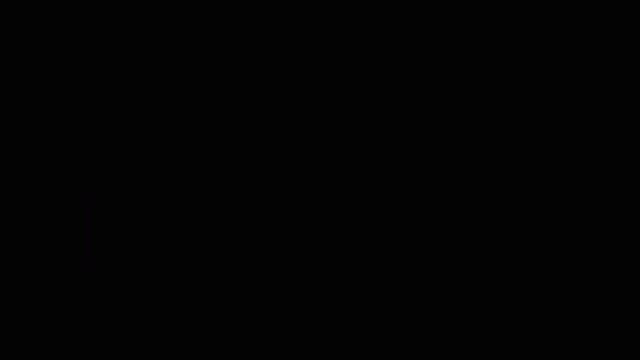 And, as always, times u prime. Now, the next two that you need to know Are the derivative of secant And the derivative of secant's cousin, Or cosecant, And they're quite similar If there's a c in front. 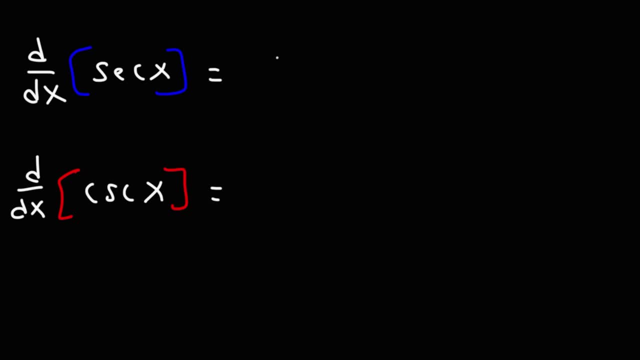 Typically it's going to have a negative sign. The derivative of secant Is. You know what? let's change this. Let's change it from x to a, u. The derivative of secant u Is going to be secant u. 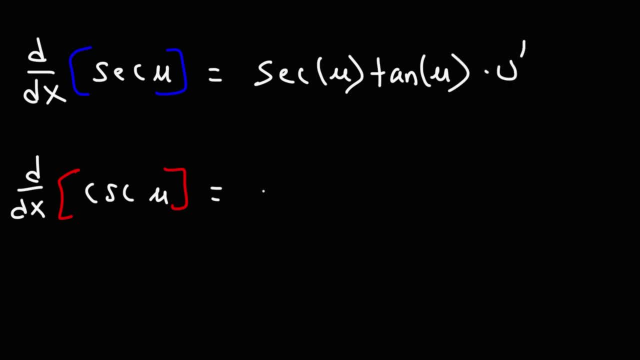 Tangent u Times u prime. The derivative of cosecant u Is negative. cosecant u- Cotangent u Times u prime. Now, the next set of formulas you need to be familiar with Are the inverse trig formulas. So let's start with the derivative. 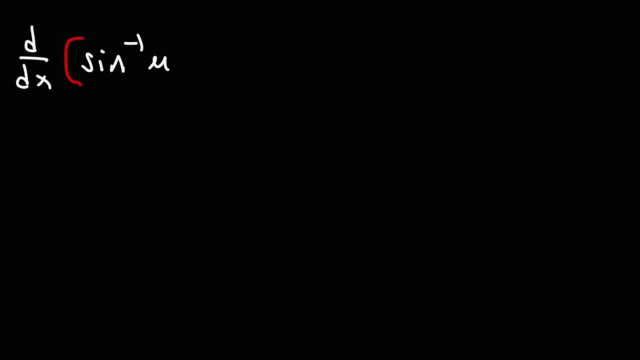 Of the inverse of sine of u. So that's u prime Over the square root of 1 minus u squared. Now just for comparison purposes, If you have the inverse sine of x, It's going to be 1 over the square root. 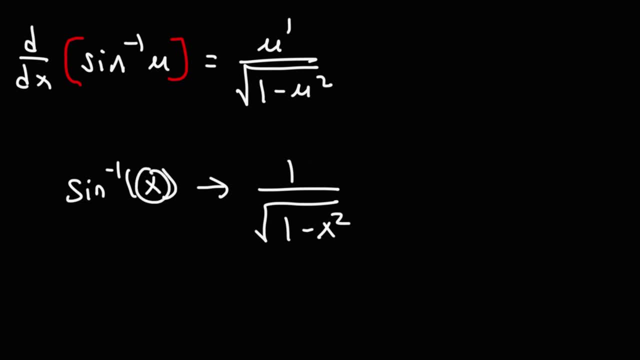 Of 1 minus x squared, Because the derivative of x is 1.. You're going to have that there. But if you have u, You're going to have u prime instead of 1.. So make sure you're mindful Of that difference. 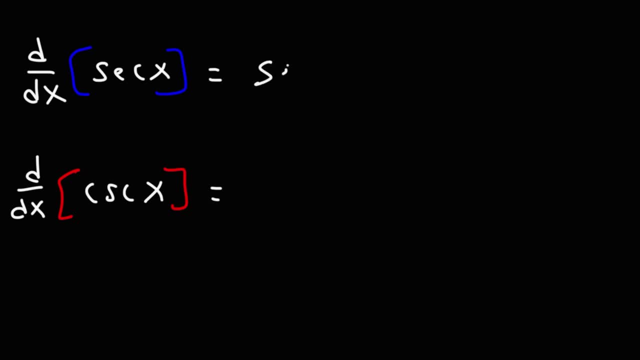 The derivative of secant is. you know what? let's change this. Let's change it from x to a? u. The derivative of secant u is going to be secant u- tangent u times u prime. The derivative of cosecant u is negative: cosecant u- cotangent u times u prime. 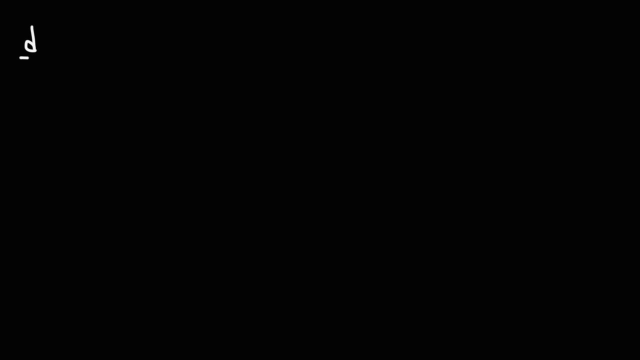 Now the next set of formulas you need to be familiar with are the inverse trig form. So let's start with the derivative of the inverse of sine of u, So that's u prime over the square root of 1 minus u squared. 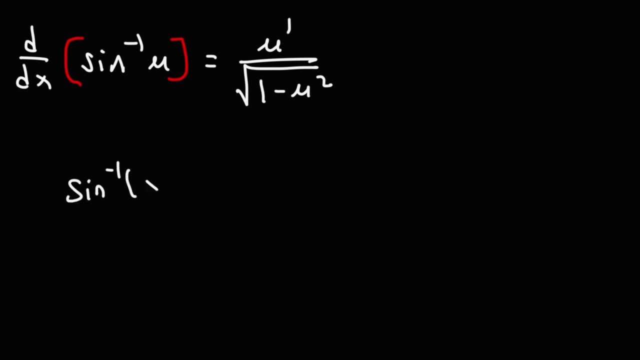 Now just for comparison purposes: if you have the inverse sine of x, it's going to be 1 over the square root of 1 minus x squared, Because the derivative of cosecant is negative sine of u. So if the derivative of x is 1, you're going to have that there. 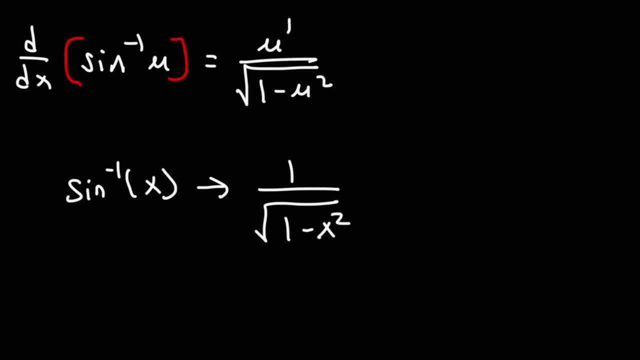 But if you have u, you're going to have u prime instead of 1. So make sure you're mindful of that difference. Now the derivative for the inverse cosine of u is going to be very similar to the derivative of sine. 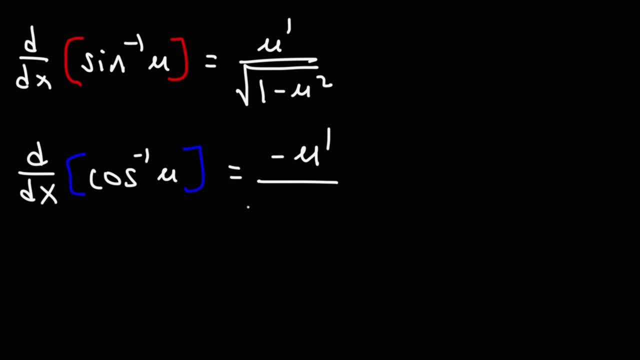 The only difference is it's going to have a negative sine, But everything else is going to be the same. So the derivative of inverse tan of u is going to be u prime over 1 plus u squared. So that's u prime over 1 plus u squared. 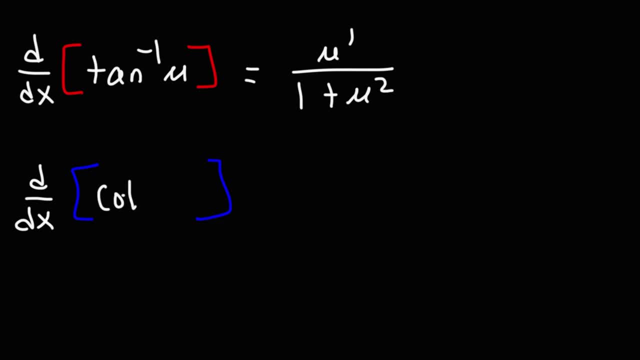 Now for arc cotangent. it's going to be negative: u prime over 1 plus u squared. Next up, we have inverse secant And the formula for that is going to be u prime. So it's going to be u prime over u square root, u squared minus 1..